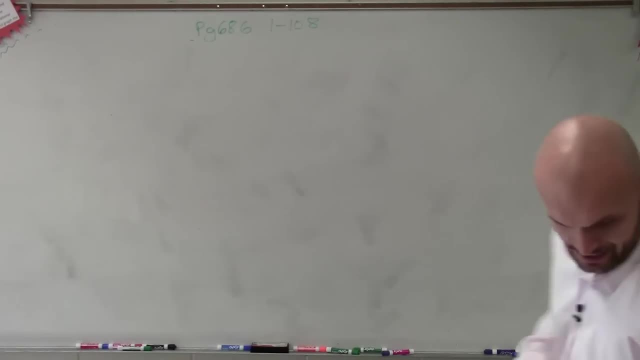 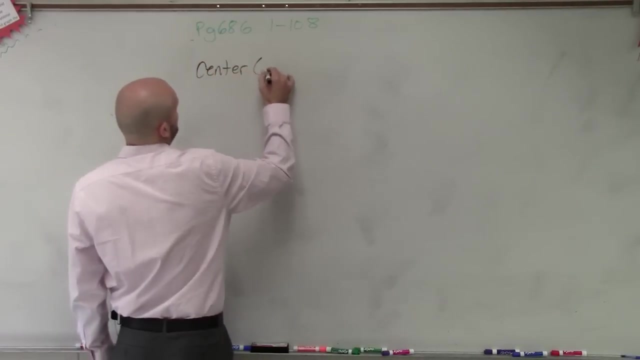 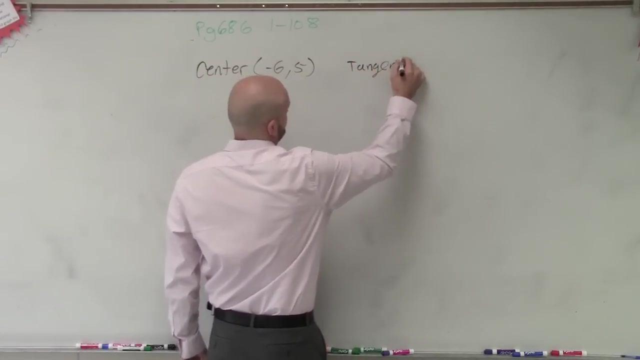 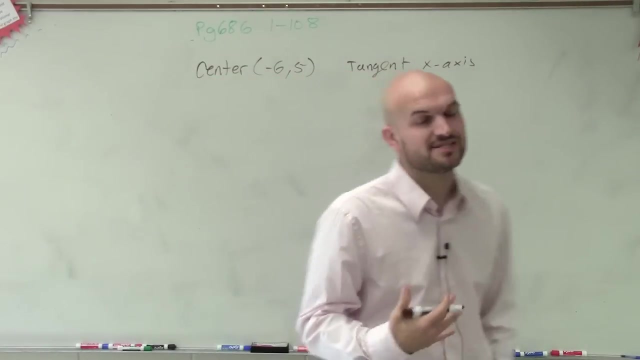 Hello, Hello, Okay, What we have in this problem is we have a center at negative 6, 5.. And we know that the circle is going to be tangent to the x-axis. All right, So first of all, ladies and gentlemen, when creating a circle, we need to make sure we go back to and at least write it in our standard form, right? 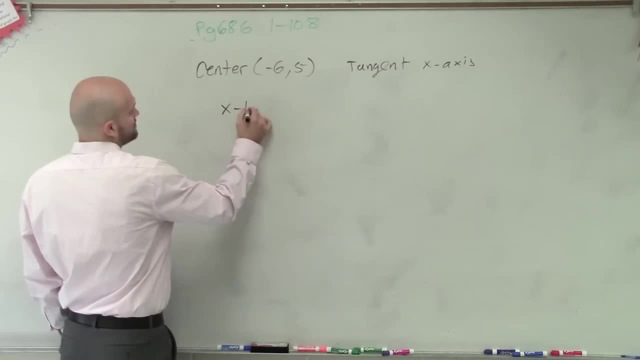 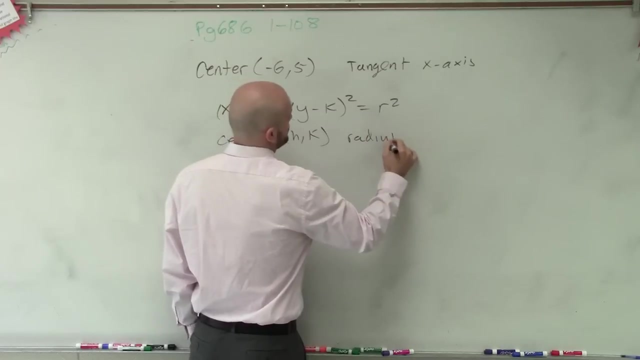 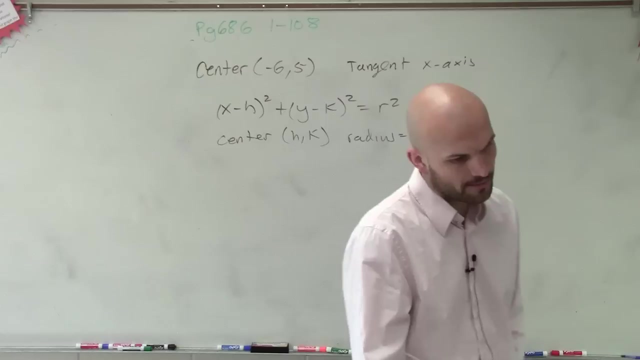 So we know that a circle can be written in standard form of x minus h squared plus y minus k squared equals r squared right, Where the center is h, comma k and the radius is equal to r, right. Okay, So all they're asking us to do is to so to write the equation of the circle. Well, we know what the center is right, And remember it's x. 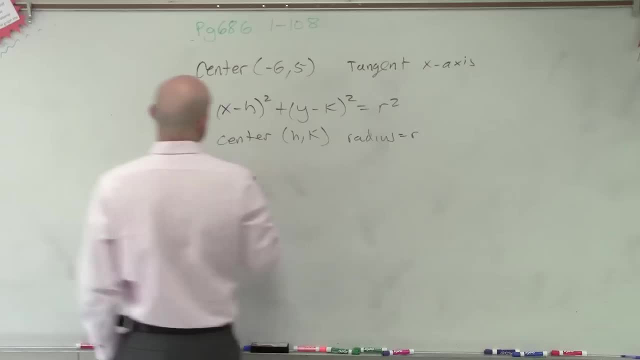 It's the opposite of h and y opposite of k. So our equation here is going to be x opposite of negative 6.. So it's going to be x plus 6 squared plus y opposite of 5, which is going to be y minus 5 squared equals. now we've got to determine what r squared is. 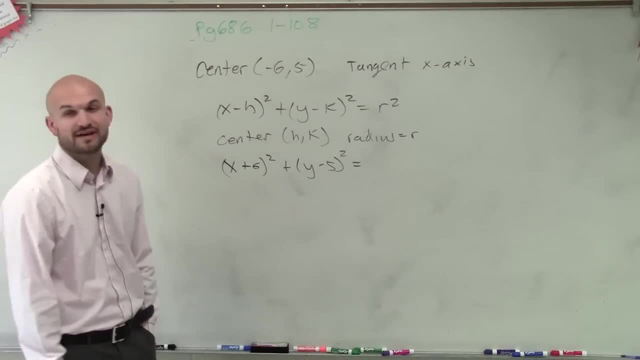 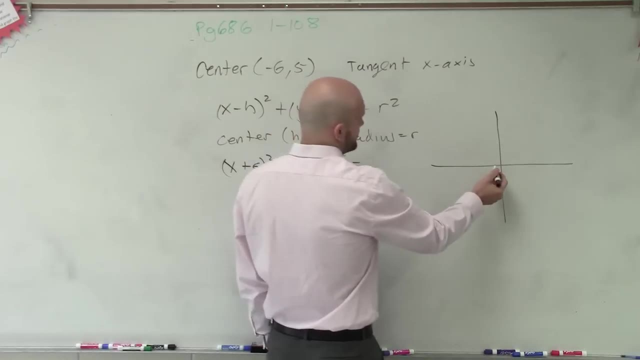 So to do that, I need to first understand what tangent to the x-axis is and what our graph is going to look like. So let me just plot this out real quick. So it's negative 6 up 5.. 1,, 2,, 3,, 4,, 5, 6.. 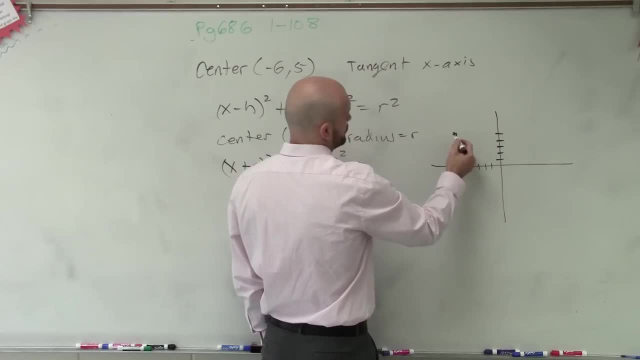 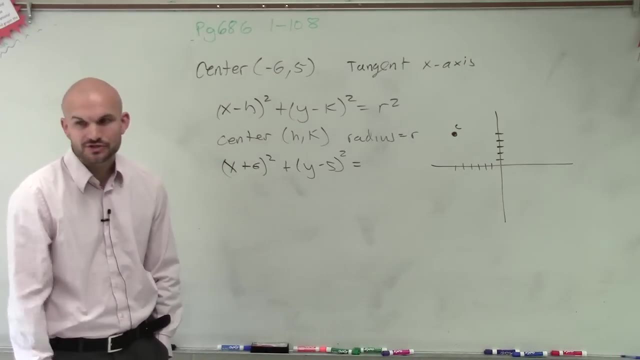 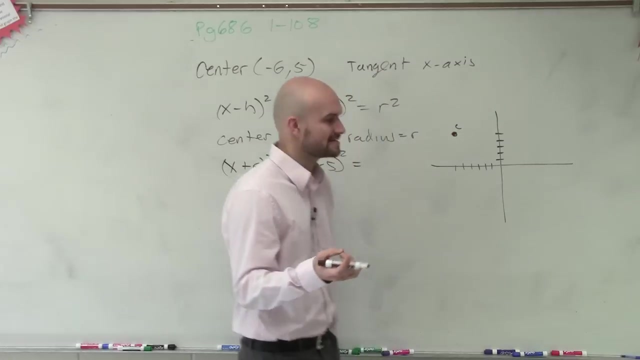 Up 5.. 1,, 2,, 3,, 4,, 5.. Okay, So roughly, my center is right there. Okay. Now, what they mean by tangent to the x-axis- all right is- means that it's going to touch at exactly one point, at the x-axis. 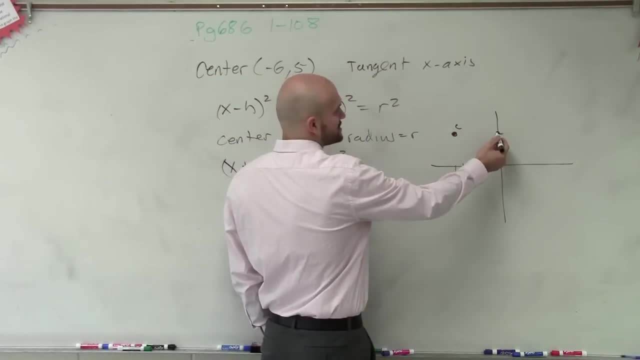 So if I was going to graph a circle, I know that it's going to tangent to the x-axis, means that it touches at that one point. All right, So if you look at like a circle, so if I was going to draw a circle here,